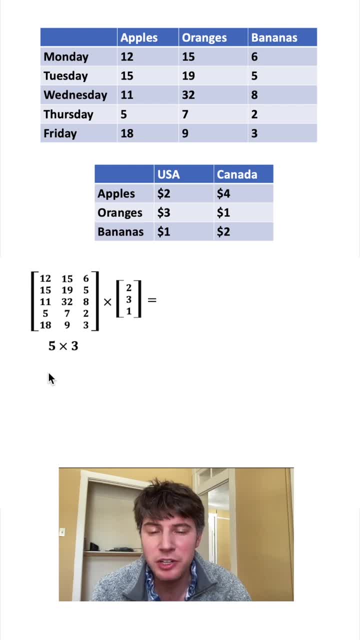 this matrix has five rows and three columns, so it's a five by three matrix. And this has three rows and one column, so it's a three by one matrix. Since these two threes match, we're allowed to multiply these And our new matrix will be a five by one, so I'll have five rows and one column. 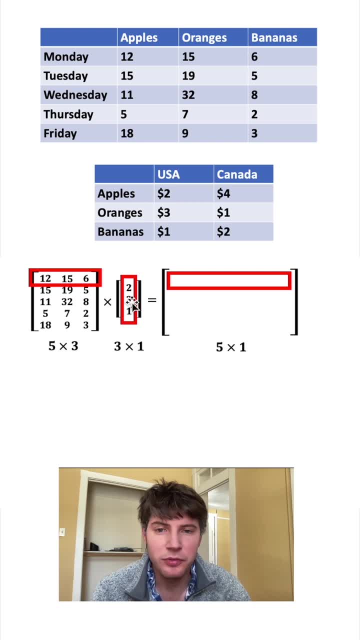 This first entry is going to be the first row by the first column, So we do 12 times 2 plus 15 times 2.. This next entry is going to be the second row times the first column, So we have the 15 times. 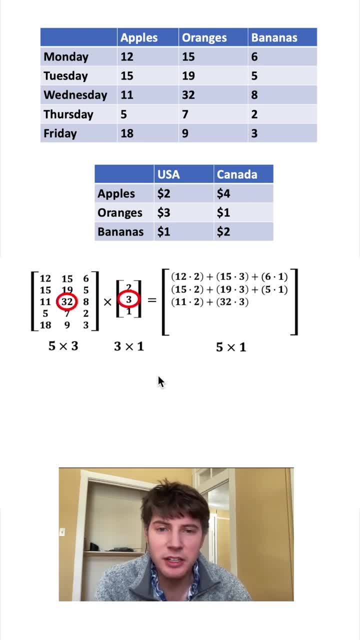 the 2, 19 times the 3, and the 5 times the 1.. And we're going to continue doing this to fill out the rest of these pieces in each of these entries. After we simplify all this, this is the matrix. 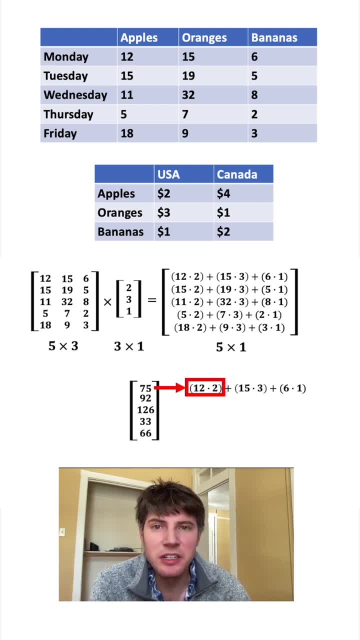 that we get. So what does this mean? This 12 times 2, this was the number of apples I sold on Monday- times the price per apple. This 15 times 3 was the number of oranges I sold on Monday times the price per orange. And this 6 times 1 was the number of apples I sold on Monday times the price per. 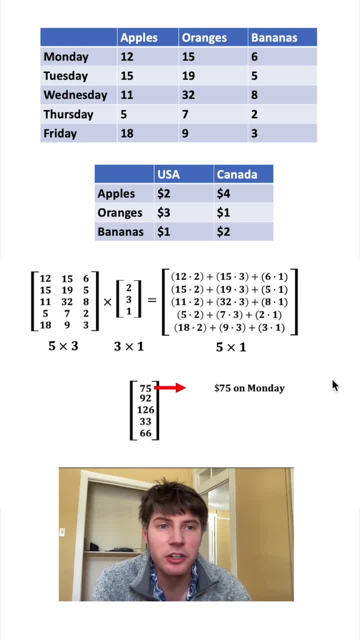 banana. So this is the $75 I made on Monday at my store, And that's what all of these are. This whole matrix is just telling me how much money I made per day at my store, And this is a real-life example of how matrix multiplication can work. Similarly, if we copy these down and then we 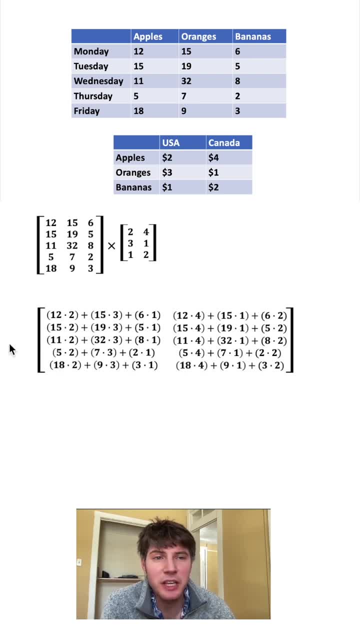 added Canada to the second matrix. we can still do this multiplication. It looks like this. And when we simplify it, it looks like this: This stuff on the left was our US sales per day. This stuff on the right would be the Canada sales per day, And we can handle way more complicated. 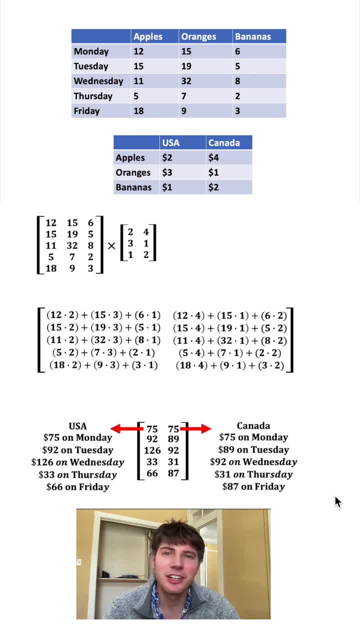 things than this using matrices. It's kind of nice. Thank you for the question. I hope you guys like this example. I'll talk to you guys soon. Bye.